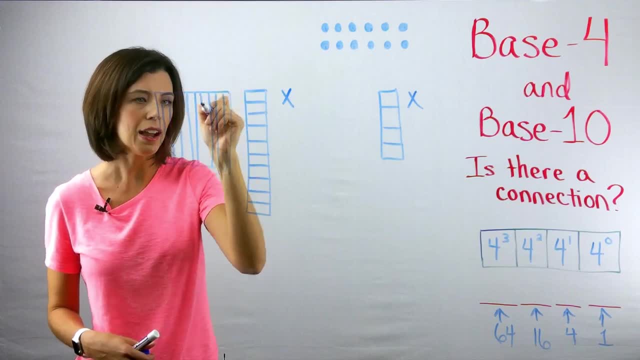 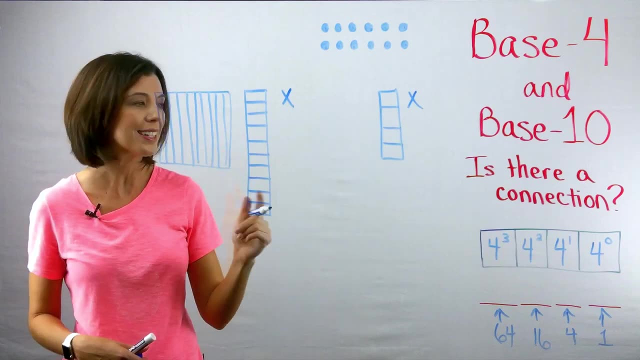 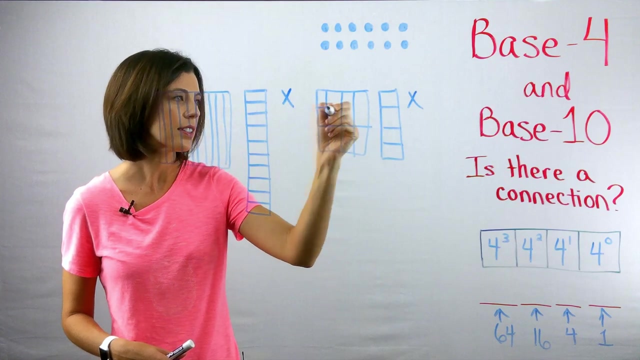 them all, but you get the picture here, okay. So it's going to have 10 of these in base four. it doesn't have 10 anymore. It has four groups of four, which would be 16.. So a flat in this case literally looks like this, Hence why we say groups of 16.. 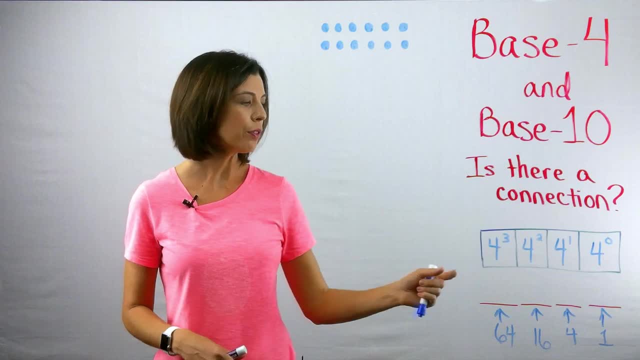 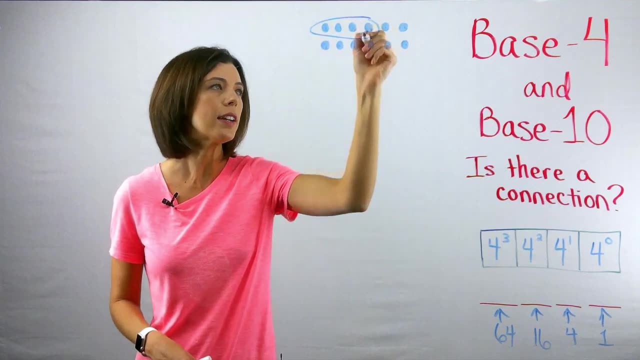 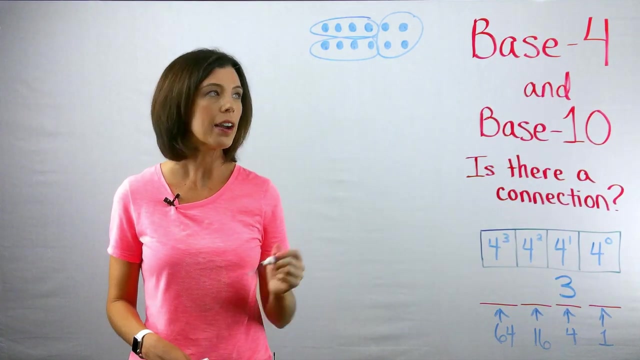 Okay, so now let's go back to our dots. We need to first see: can we count by ones We could? Can we count by groups of four? Well, let's see, I've got four here, four here here and four here. So I have three groups of four. I'm going to write a three there I have. 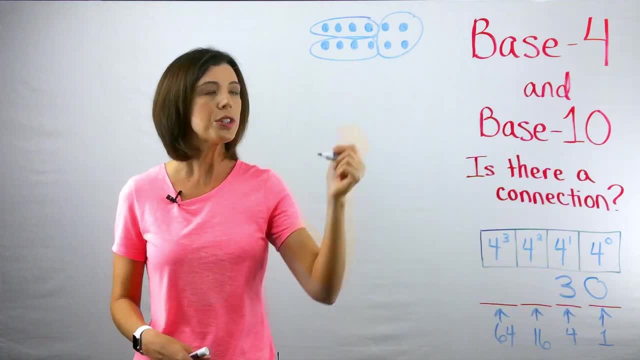 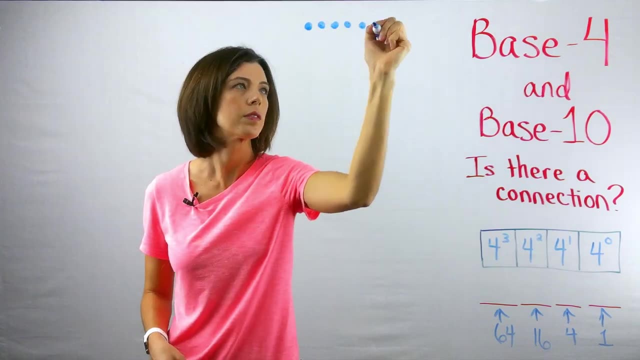 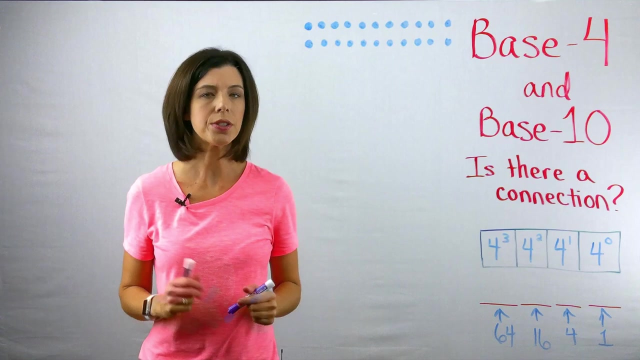 zero ones once I've grouped by fours. So this number is going to be written 30 base four. Let's try another one. So now I have this amount of dots, So let's take a look again Again, I can group by ones. 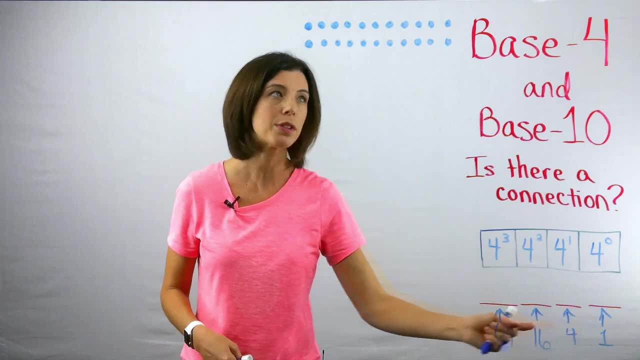 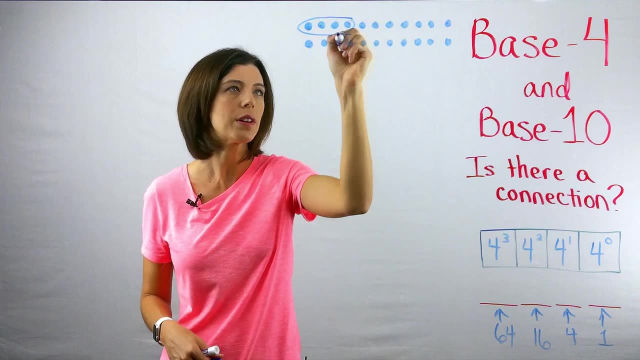 but I'm going to see that I'm going to be able to at least make groups of four. Hmm, I even noticed that maybe I can make a group of 16.. So let's let me start by fours first. So I've got four. 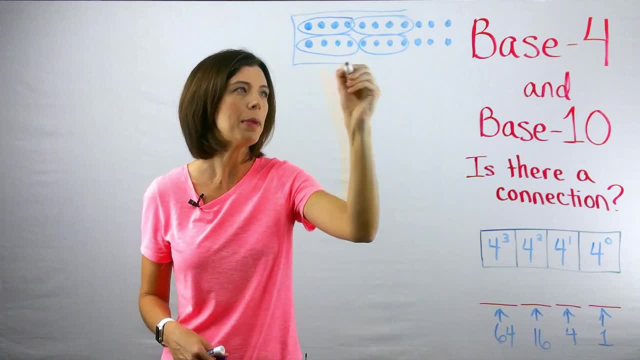 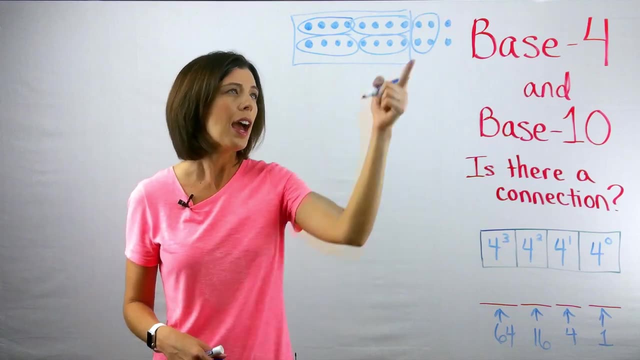 four, four, four. Okay, So I can make a group of 16 and I've got another four here and two ones. So again, let me write that down. I have one group of 16.. So I'm going to put a one there. 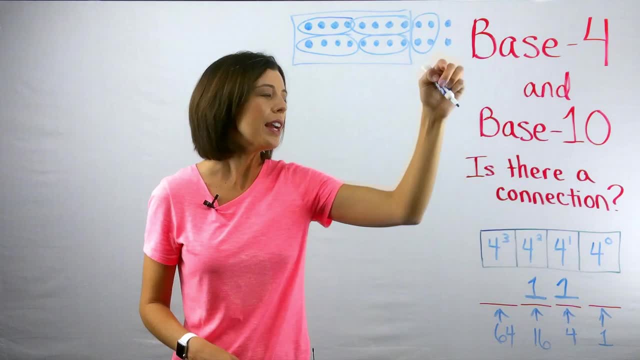 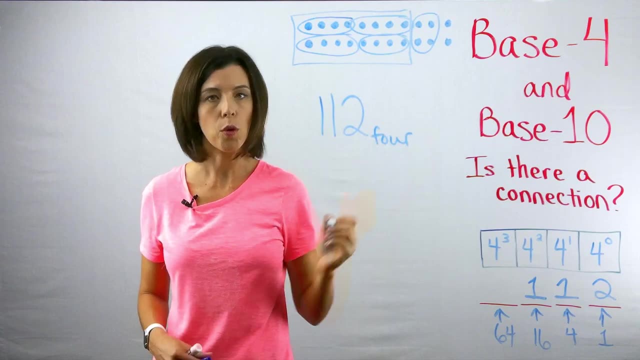 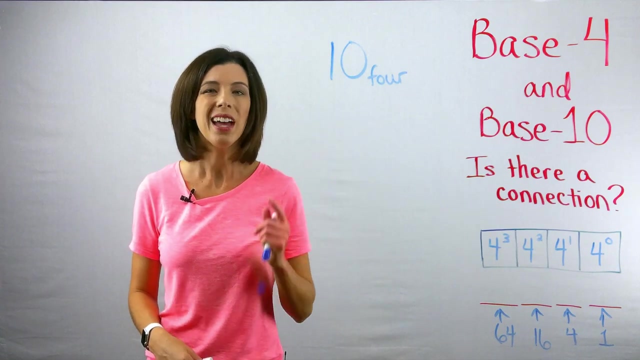 I have one group of four. I'm going to put a one there And then I have two Again. this number would be 112 base four. Now how about the questions that ask you to give the number that comes before 10 base four? The easiest way to do this, in my opinion, is to draw out your 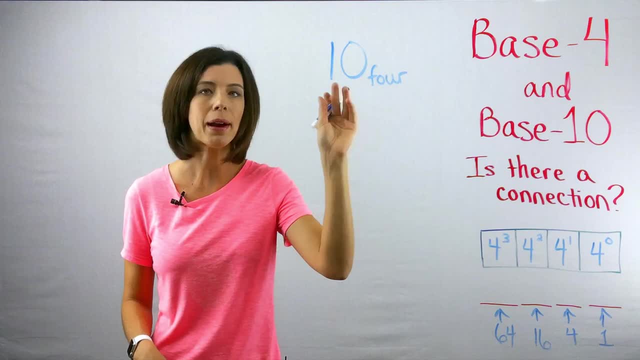 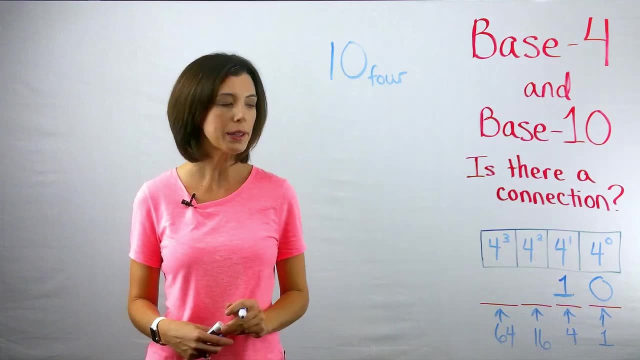 dots. So I'm going to go ahead And first of all I need to think about what, how many groups of what is this? So I'm going to go ahead and put it over here on my little base: four place value, And I see that I have zero ones in one group of four. 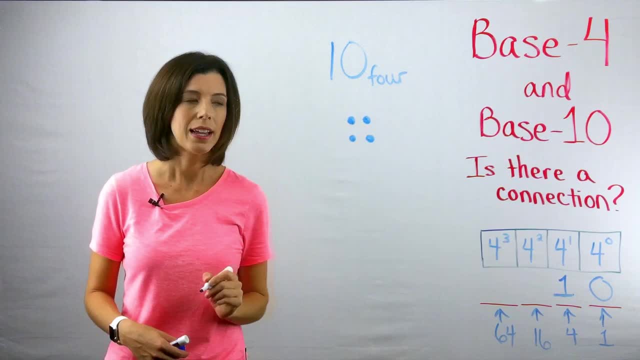 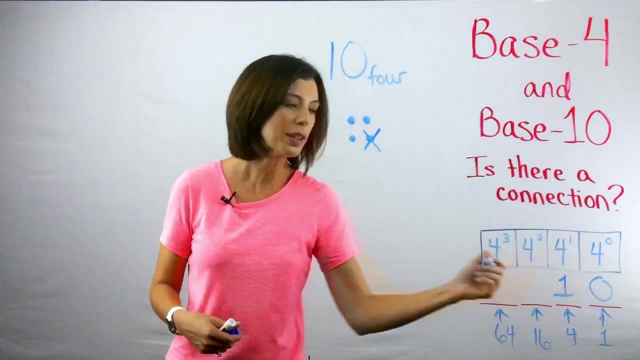 So I'm going to go ahead and draw four dots. Now, if I go ahead and take one away, I can see that I only have three units. Again, I can put a three underneath my ones here, And I know that this is. 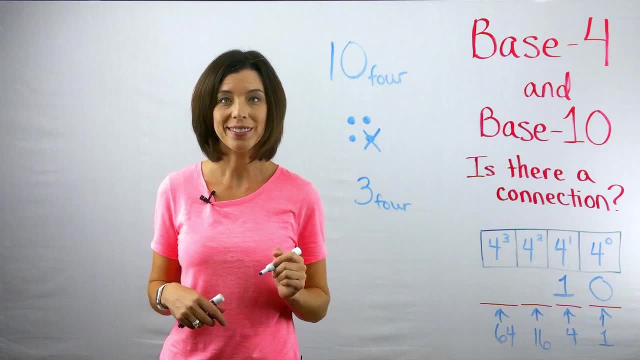 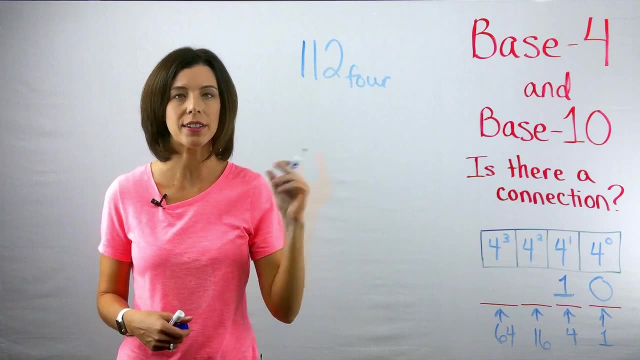 three base four. Let's try another one. Let's think about what's the number that comes before 112, base four. So we just kind of looked at these dots. Let's go ahead and take it apart. If I go ahead- and again I'm going to think of this as 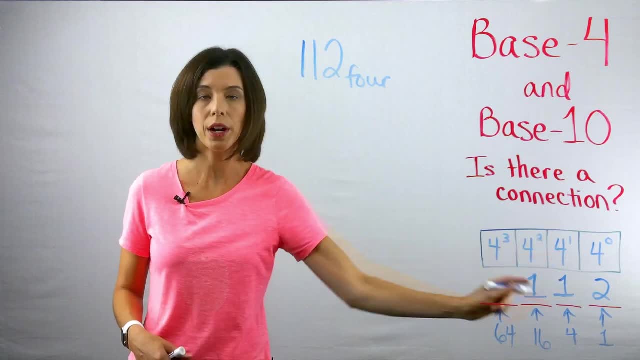 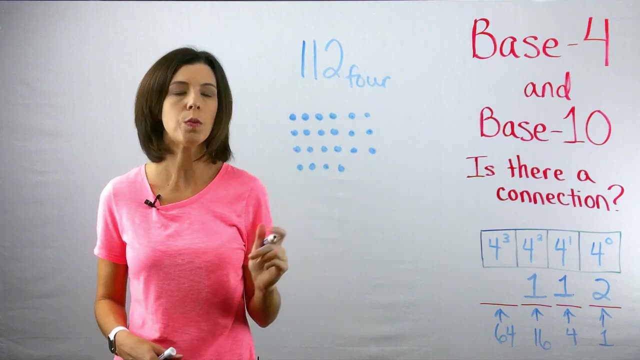 one group of 16, one group of four and two ones. I'm going to go ahead and draw that Now. I have one group of 16, one group of four, two ones. If I get rid of one now, let's see what I can. 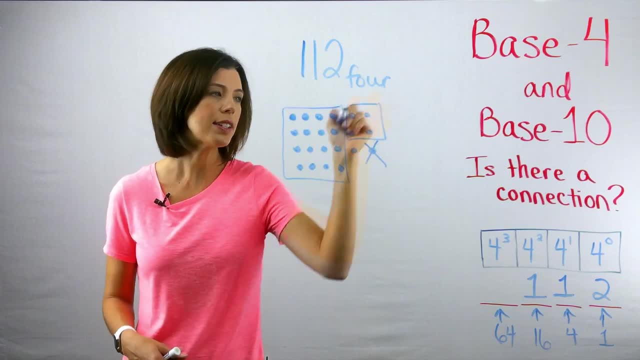 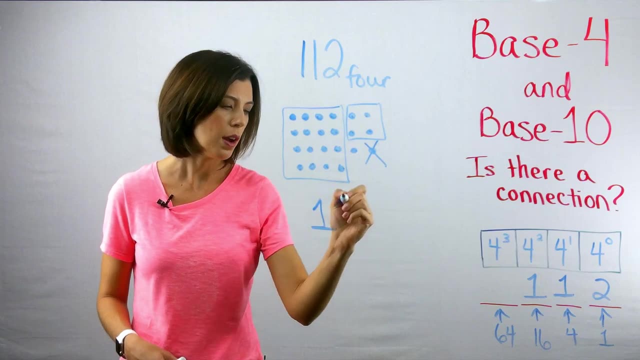 group. I can still group my group of 16.. I can still group my group of four. So I'm actually going to have one group of 16, one group of four and one one, So 111 base four. What if I wanted to? 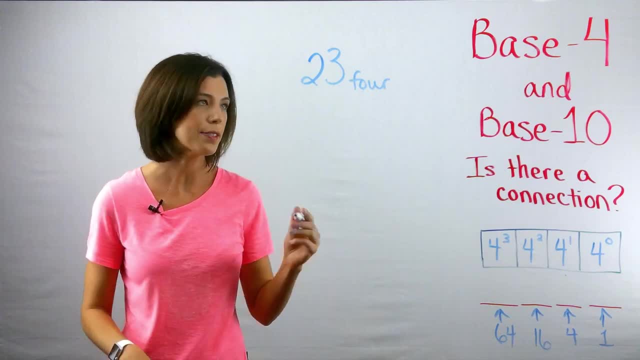 think of the number that comes before 10, base four. I'm going to go ahead and draw that. So I'm going to think of the number that comes after this. Let's plug it into our place value chart. So again, I have. 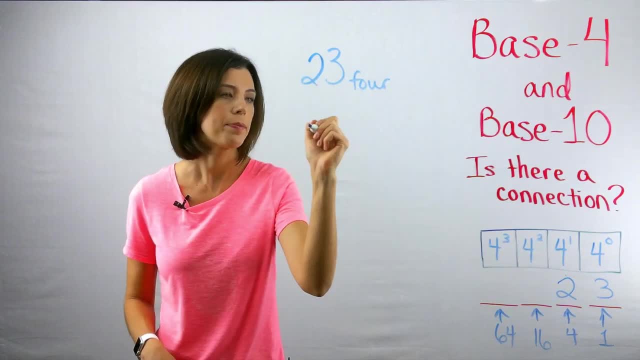 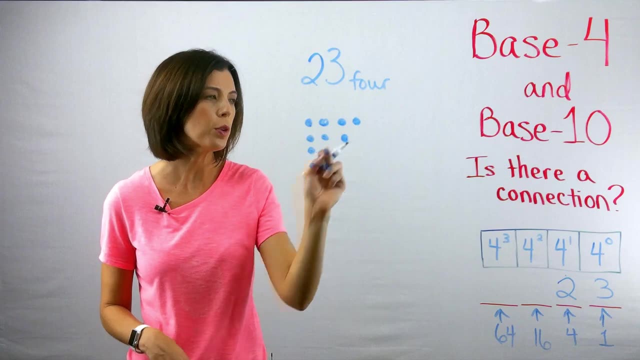 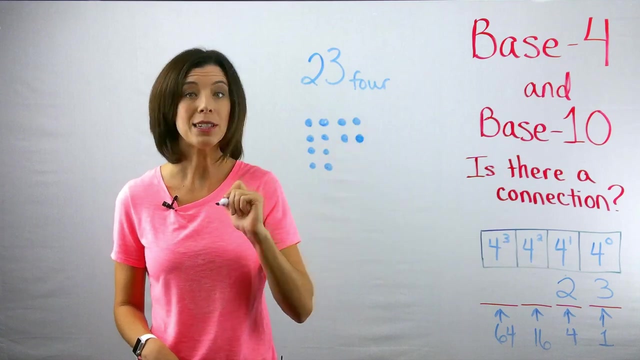 three ones, two groups of four. I'm going to draw that. So I have two groups of four. Okay, so now you can see I have two groups of four, three ones. If I add one more on, I've added that one on. Now let me circle my groups of four. I have one, two, three. Now I have 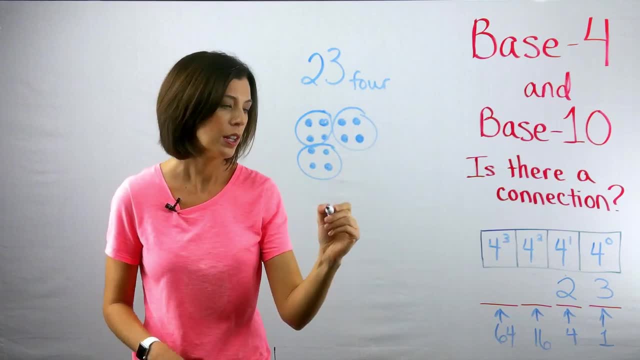 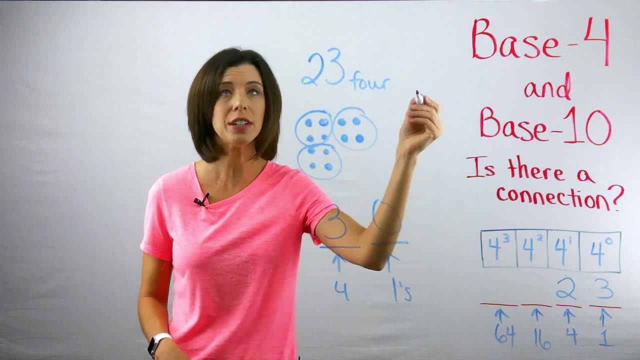 three groups of four and zero. So I have one, two, three. Now I have two groups of four and zero ones. So I have three groups of four and zero ones. This number, the number that comes after this, would be 30 base four. That would be the number that comes next. So I hope you have a. 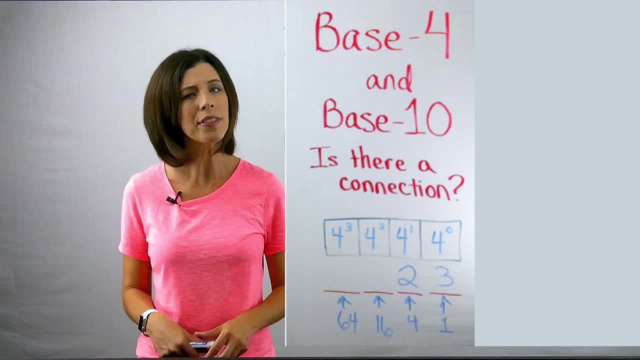 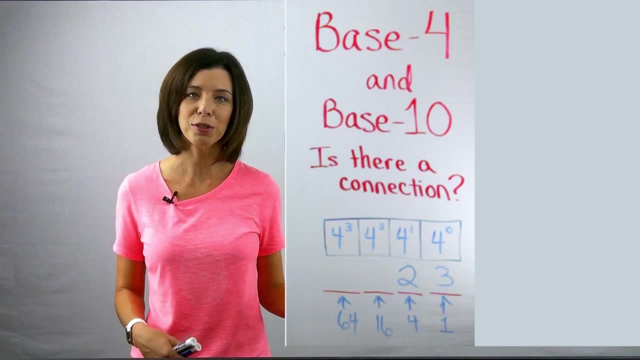 better understanding now of other base math. Stick with it. Persevere. This is not something really easy to think about. Know that, because this is not natural for you. we don't operate in base three, We don't operate in base four, We operate in base 10 world. So just know that. 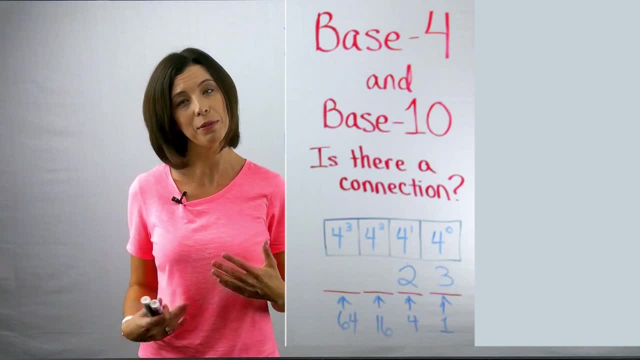 your students are going to struggle with base 10, just like you're struggling with base three or base four. Have a great rest of your day.